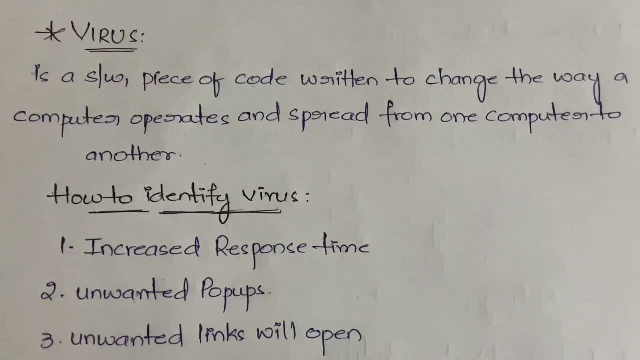 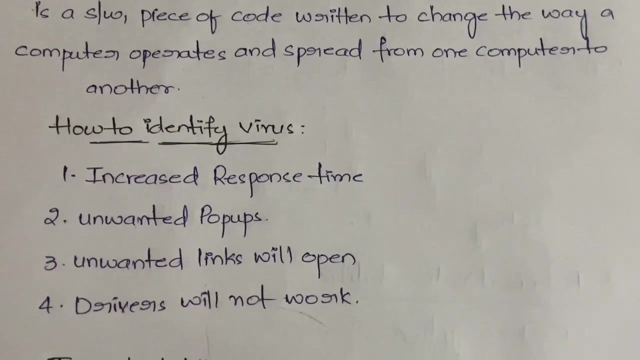 And all. But if camera is not working properly, instead of doing clicking pictures, or instead of using it for video call, it is doing something else, Then it has a virus. Same with the calculator as well. So what is the actual function? Instead of doing that, it is doing something else. Then a virus is infected. Okay, and how do you identify the virus? So first is in increased response time. For example, you are opening an application, Then it. 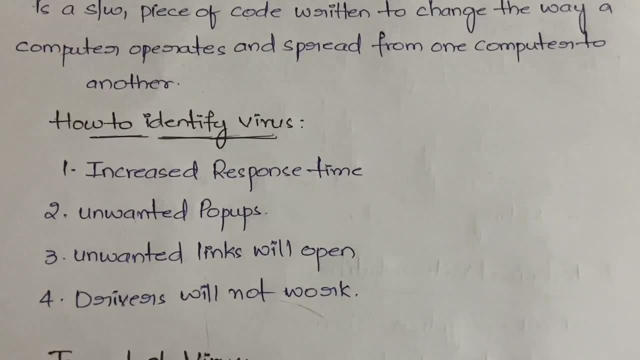 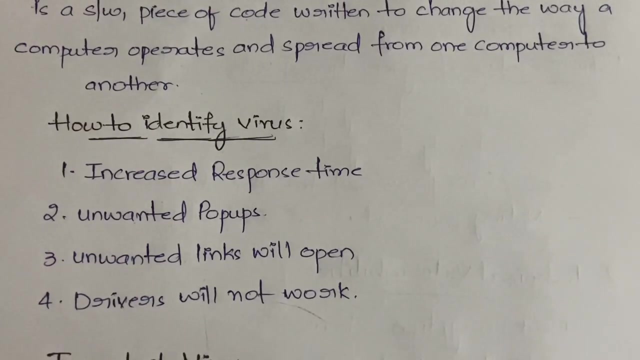 has to open within 10 seconds or 30 seconds max, But more time. if it is taking, it means some virus is there. Response time is increasing. Next is unwanted pop-ups. You will be getting all unwanted pop-ups Always. you will be getting. So that is no way related to you, but you will be getting it And unwanted links will open. So, particularly when you are using some websites to download movies automatically, some unwanted links will be opening in the new tab Right So that and drive. 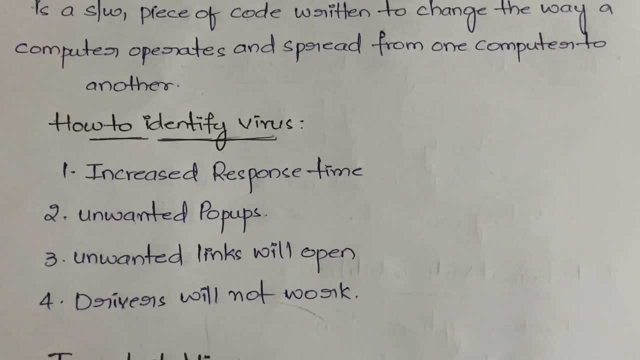 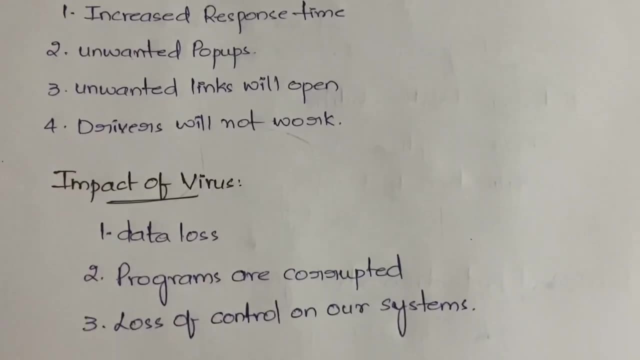 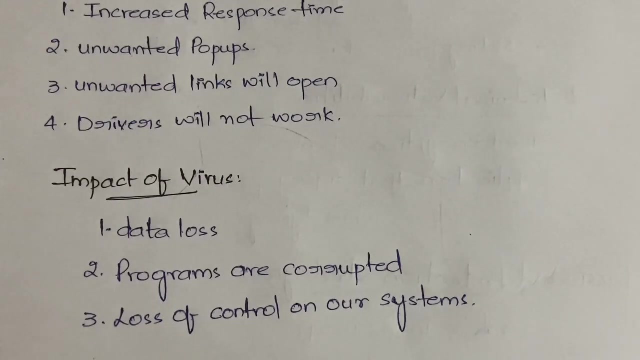 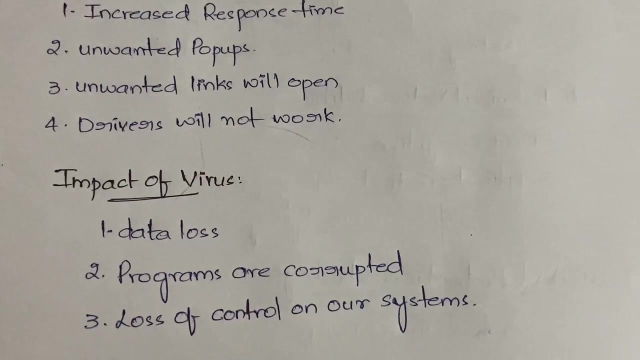 drivers will not work. Drivers- different drivers, we have in our computer, Right? So any of that driver or all the drivers may not work properly. Okay, Next is impact of virus. So how a virus can affect you, What a virus can do to your system. Data loss: Our data can be lost: Our contacts or photos or movies, or any files. they can be lost And programs are corrupted. That is why, if programs are corrupted, only then the functionality will change, Right. 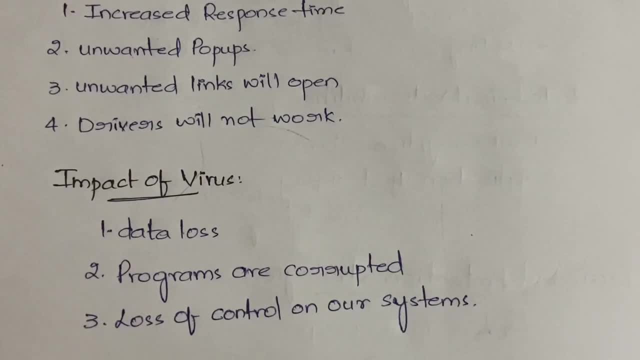 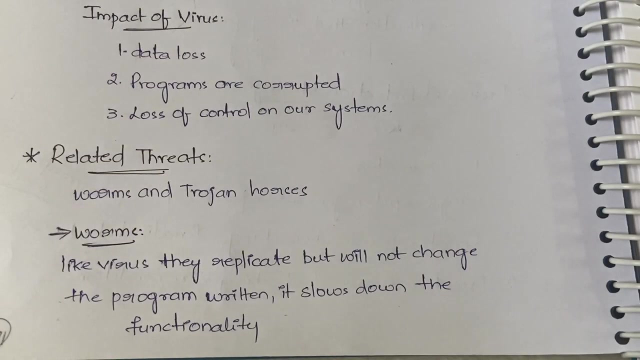 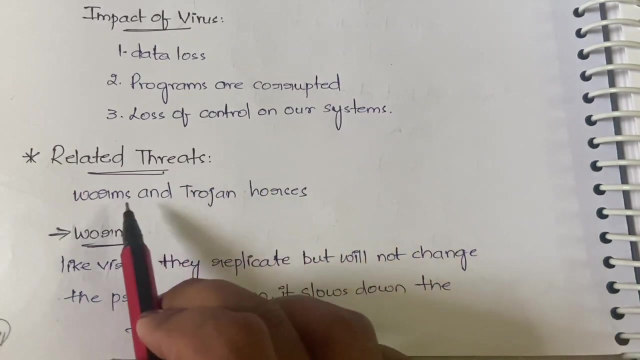 Next, loss of control on our system. On our system, we will be losing our control, So what is happening in our system will not be in our control. You are clicking something with the mouse, but something is happening like that. Okay, Yeah. So now let us see what are the related threats and how, what are the countermeasures and what to do So first, the related threats to virus are worms and Trojan horses. Worms and Trojan horses are also similar to virus Like. they will also affect you. 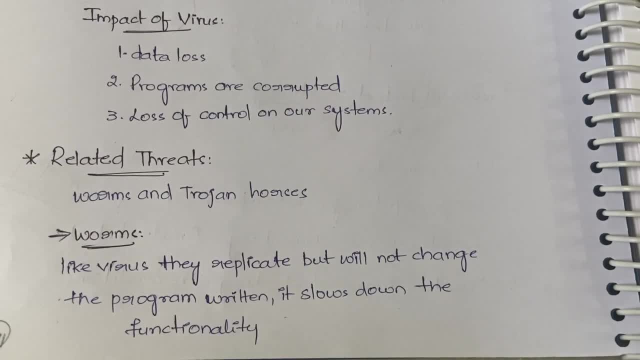 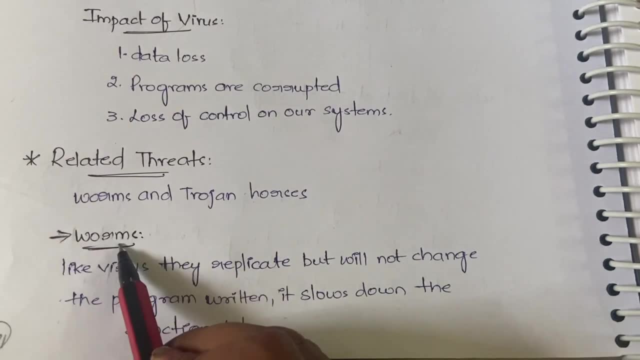 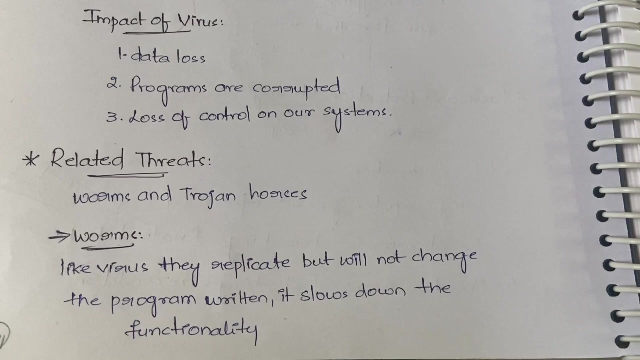 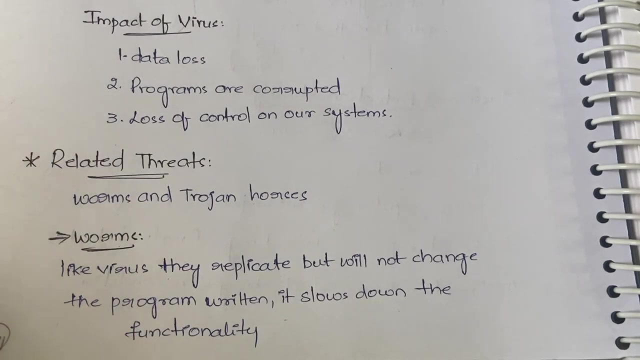 They will also affect our system. They will also disturb the functionality of our system. How, Let us see how worms and Trojans are different from virus. Let us see. So, basically, worm is nothing, but it is also like virus. It will replicate. Replicate in the sense, if, suppose, one virus for same, like coronavirus, if, if one unit of virus has entered our body, it will replicate, that is, it will multiply by itself, and so many virus particles will be produced in our body. Right? So the 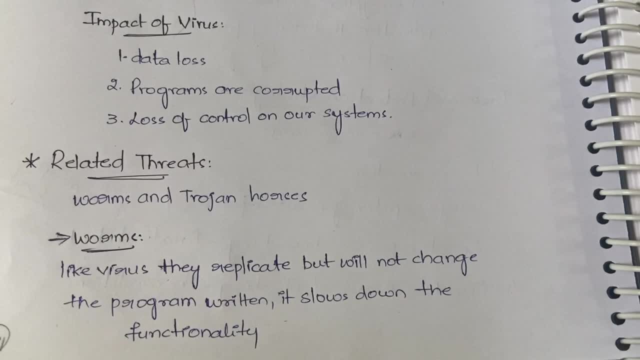 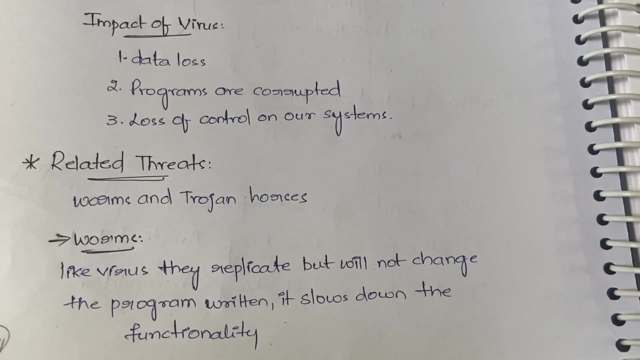 same way with worms also. So many particles will be generated. So worms like virus, they will also replicate, but they will not change the functionality or they will not change the program return. It will just slow down the functionality. So what virus is doing? it will change the way in which the computer operates, Right, Virus? what virus is doing? Suppose, if suppose, if you're clicking one plus two, instead of adding one and two, it will subtract one and two. That is what virus does. 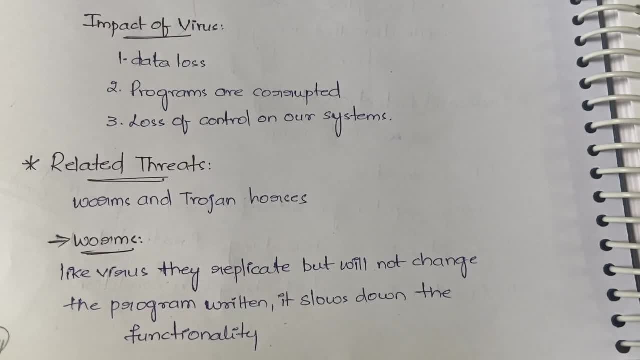 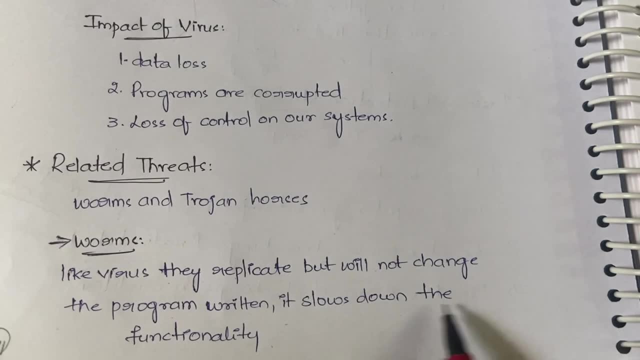 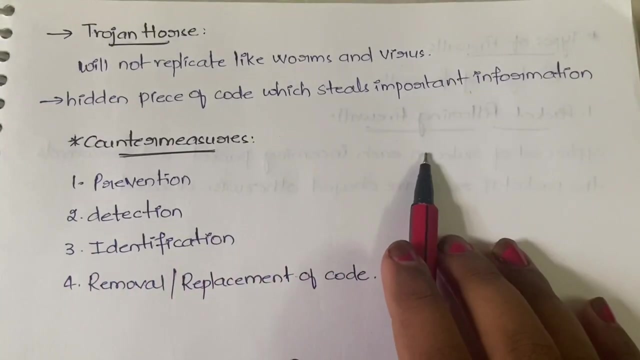 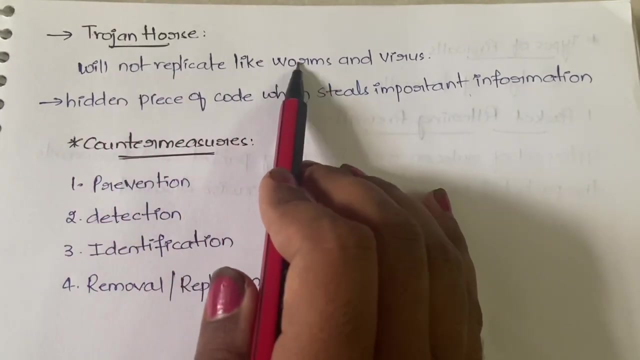 But worms will not change the functionality. Suppose, if you're clicking one plus two, one plus two only will be done, but that will happen slowly. Okay, it will just slow down the functionality of the system. It will not change the functionality of the system, Got it? You got to know what is a worm now. Now let us see what is a Trojan horse. What is the difference? now, A Trojan horse is nothing, but it will not replicate like worms or virus. That is, if once it is entered into our system, it will not replicate. 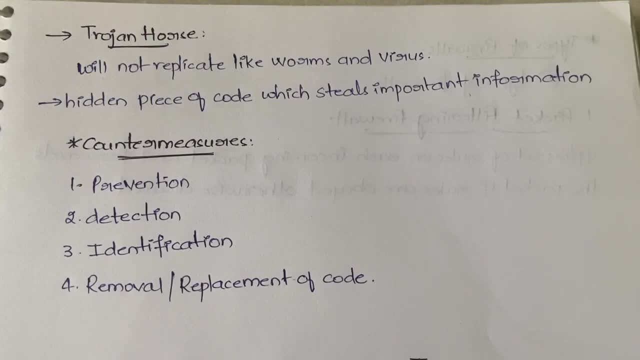 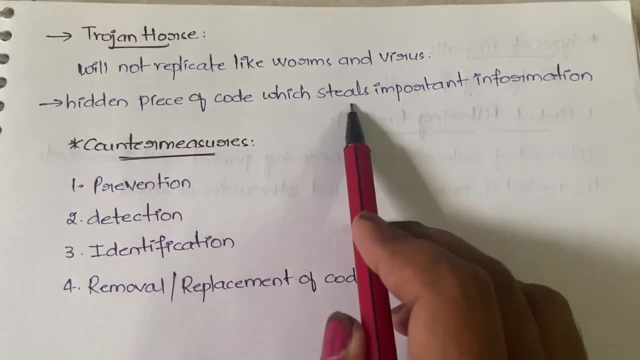 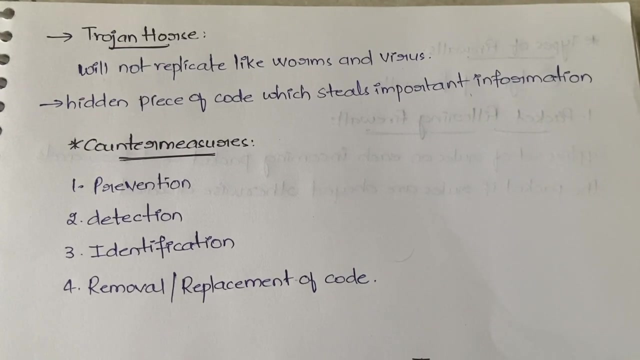 like worms or virus. worms will replicate, virus will replicate. sorry, right, but it will not. hidden piece of code. it is a hidden piece of code which will steal the important information. the important information which is present in our system is stolen. that is the. that is what the trojan horse will do, what virus will do: it will replicate and also it will change the. 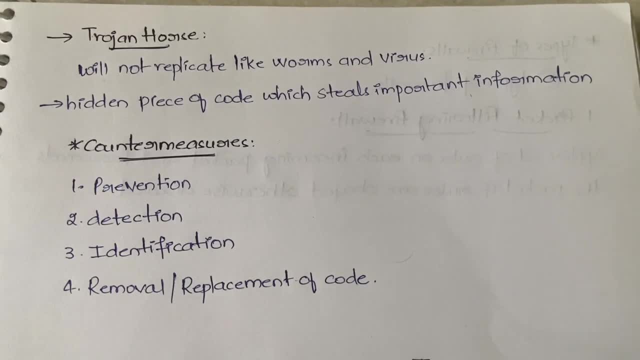 functionality right. what worm will do? it will also replicate, but it will slow down the functionality. what trojan horse is doing? it is not replicating and it is what it is doing. it is stealing the important information. got it now. what are the counter measures to it? let us see. 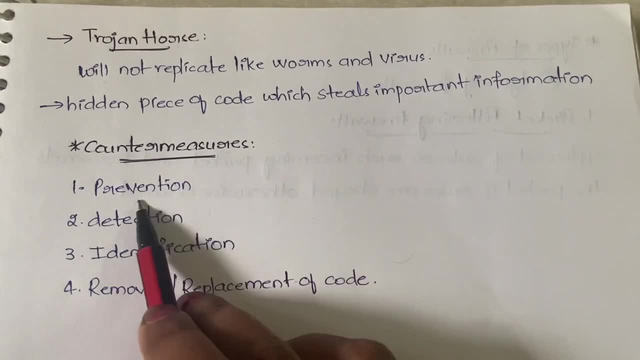 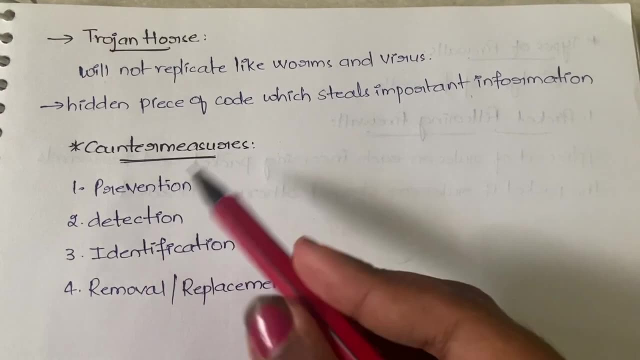 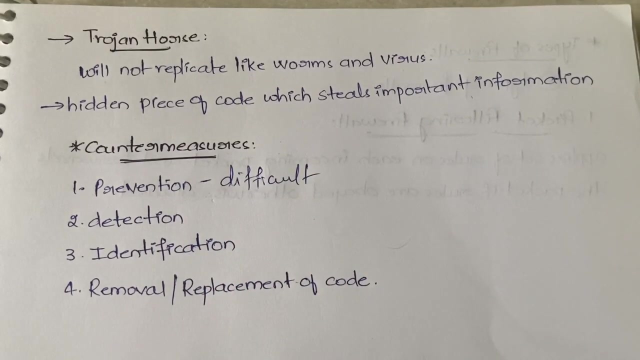 so, uh, moving to the counter measures, prevention. prevention is always better than cure, we say, right in science we have this. so prevention is always the better, the best solution. but prevention is difficult. you cannot just sit, uh, like you know. you cannot sit like a security guard right to monitor what traffic is coming into your system, right? so prevention is only. 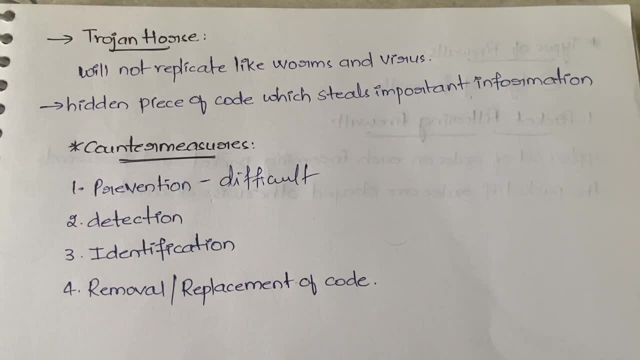 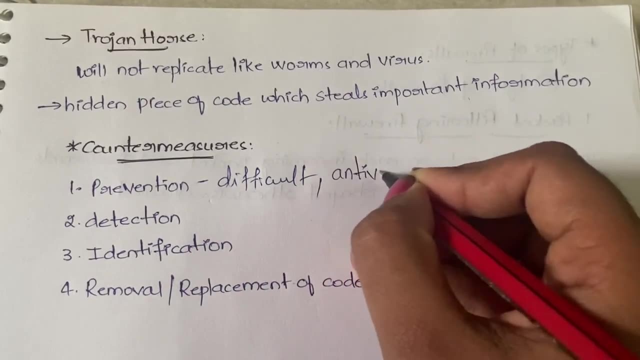 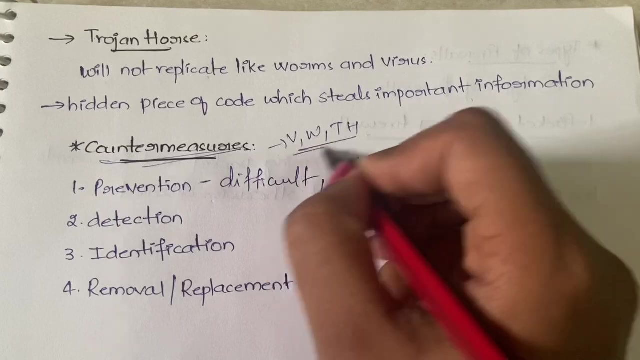 the best solution for this, but it is a bit difficult, got it. so, in order to prevent it, what you can do is you can use antivirus systems. antivirus systems okay, and these counter measures are not only for trojan horse, it is for all: virus, worms and trojan horse. okay, so you can use. 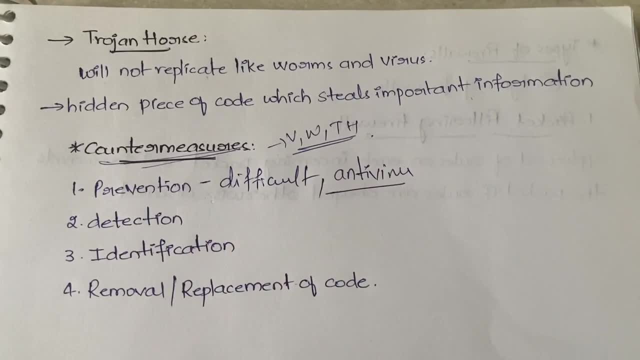 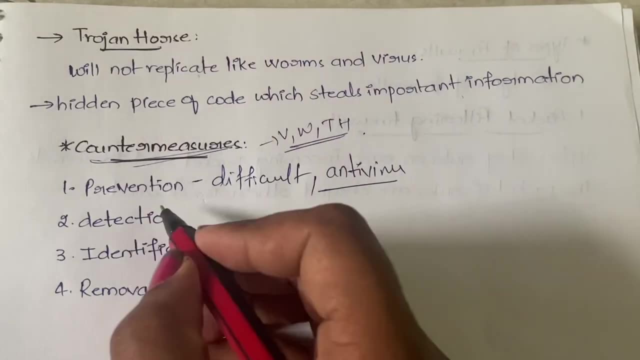 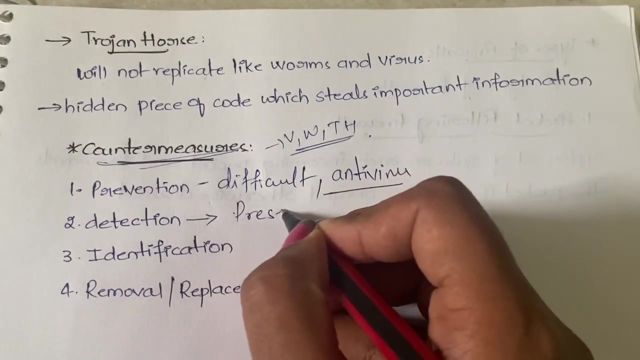 some antivirus systems in order to prevent them. even if we use antivirus systems also, sometimes some virus will enter into our system. but still we have to use detection. so detection is nothing, but you need to first detect whether the virus or whether the worm is present in your system or not. 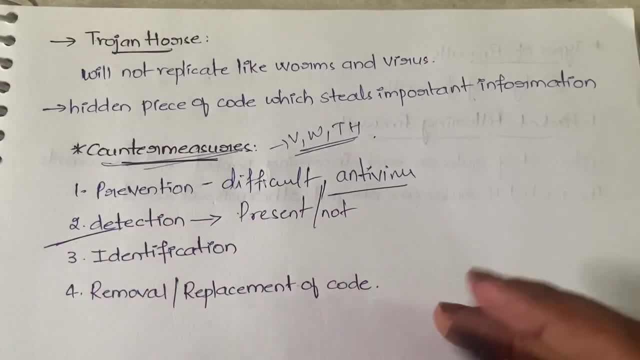 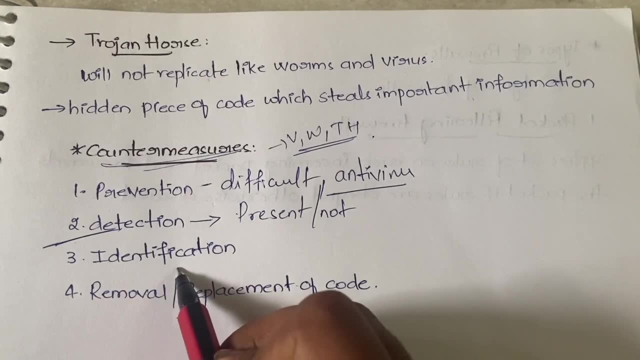 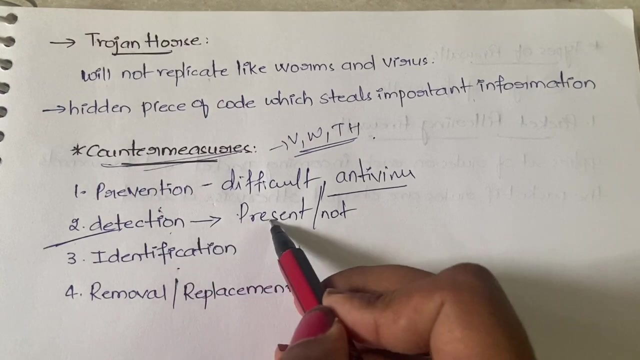 whether it is present your in your system or not. if you detect it, then you can start working in order to remove it right. you must be able to detect it. next comes the identification. identification in the sense: what is the difference between identification and detection? then detection means you will just detect whether the virus is present in your system or not. 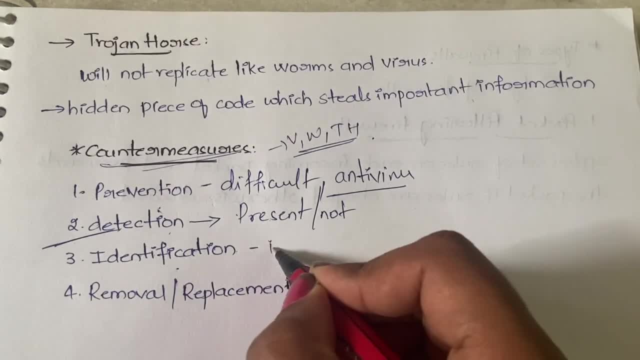 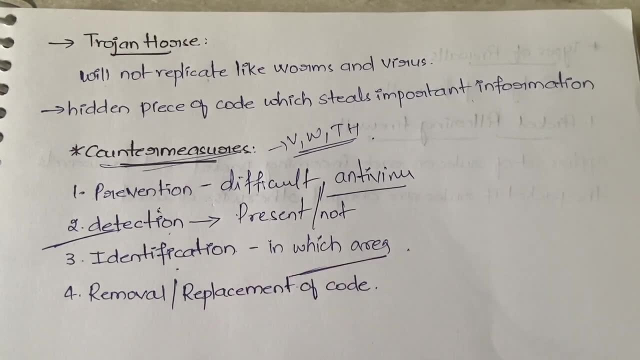 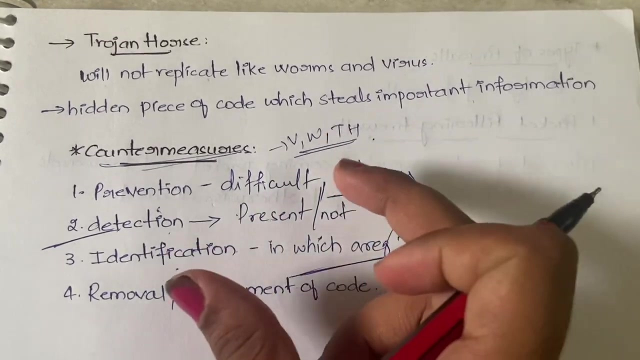 whereas identification what it will do, in which part or in which area the virus has infected- okay, in which area the virus has affected hard disk or memory or, you know, input devices or output devices or whatever it is, remote devices. whatever it is where the infection has happened. where did the virus attack the system? okay, next comes the. 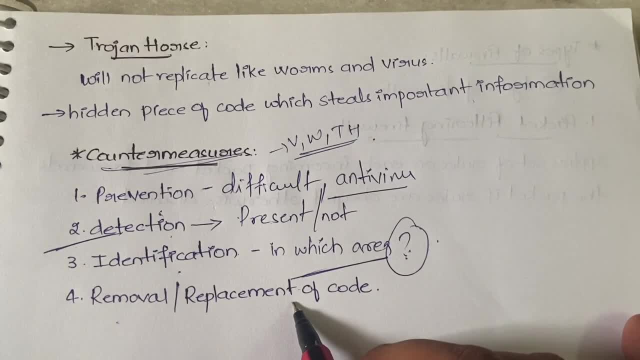 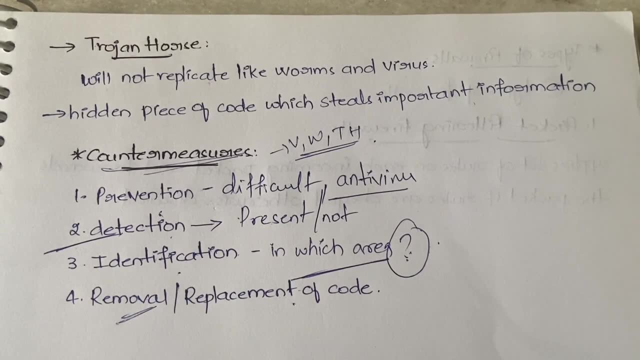 removal or replacement of code. so removal or replacement of code. removal of code is not possible. if you completely remove the code, then you cannot do that functionality again, right? so instead of removal of code, what you can do, you can replace the complete code or software with a new. 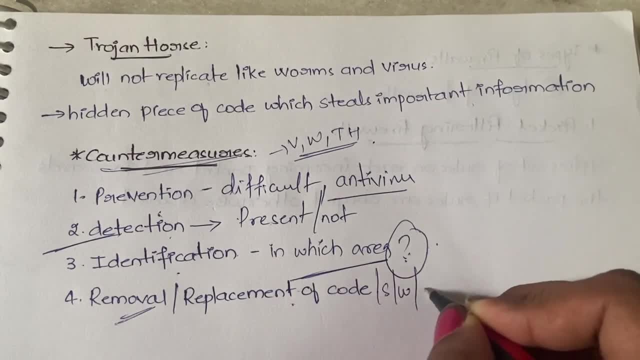 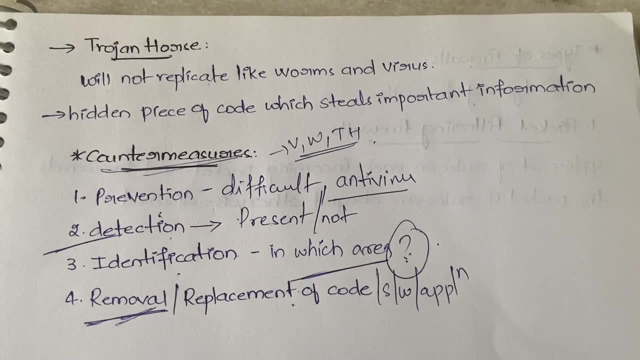